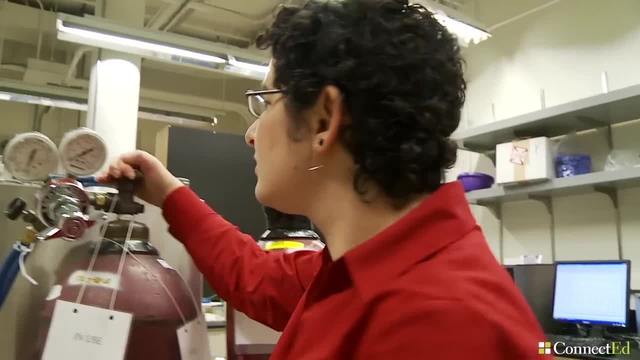 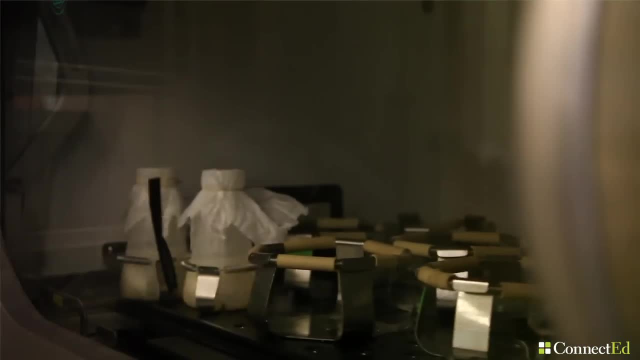 working with my hands. I like being up and doing stuff. I'm a very hands-on person. I like figuring things out and fixing them and and working with complex machinery. So I do a lot with lab robotics and automation. I do a lot with 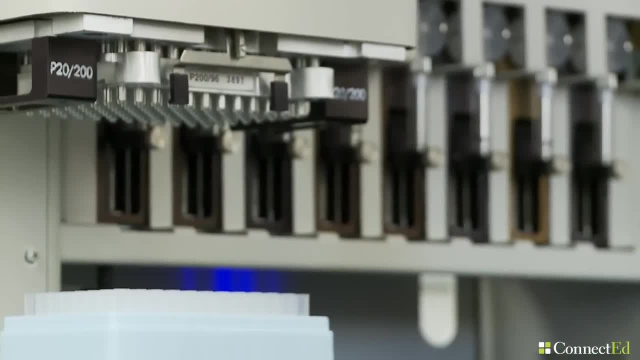 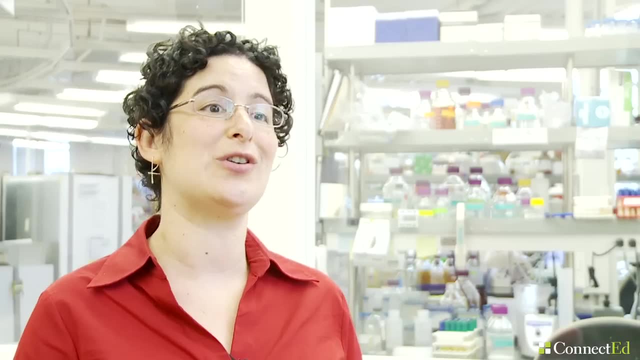 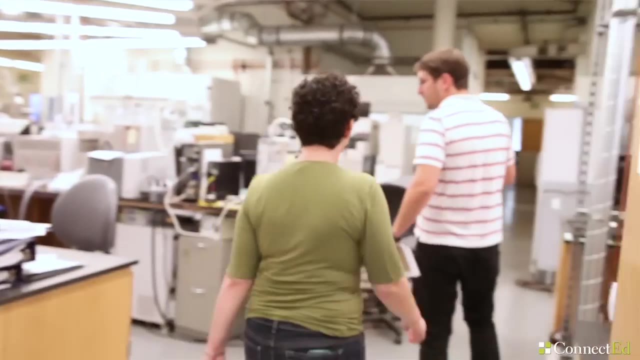 different, fairly technical things. I do a lot with robotics and I do a lot with technical instruments, So there's always stuff to learn, and that keeps it really exciting. My door is usually open and people come by when there's problems, So those problems can be this instrument isn't working or my results didn't look good. 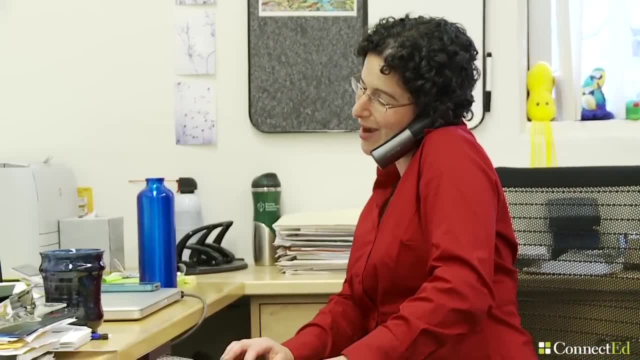 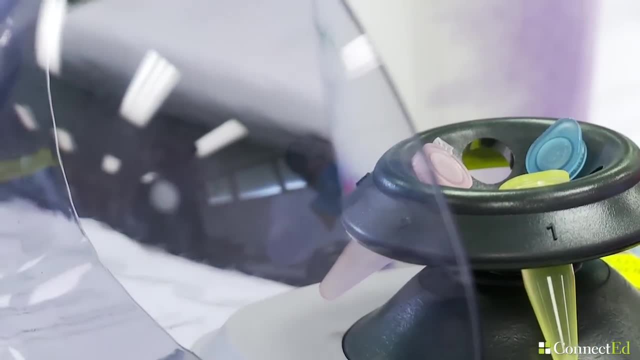 It's very, very variable and there's no real typical day, which I like. I started as a pre-med student because in high school, when you were good at biology, they told you you should go into medicine and I quickly realized that wasn't for me. 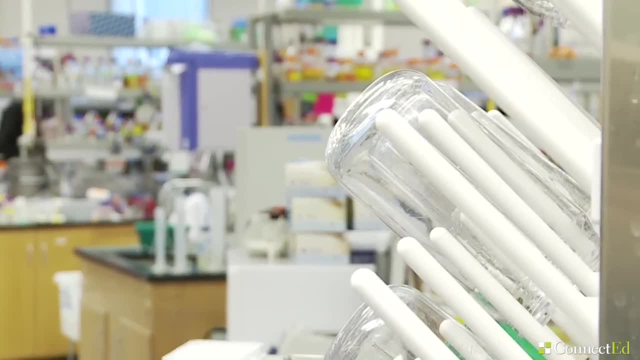 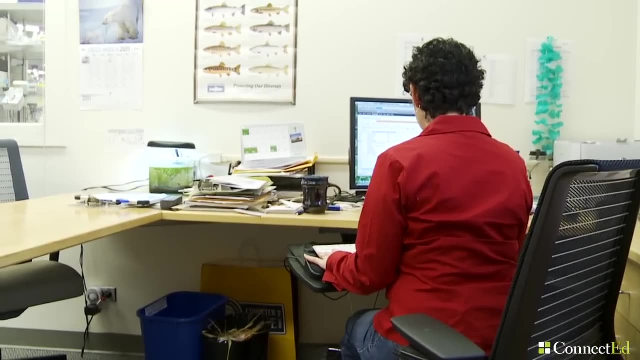 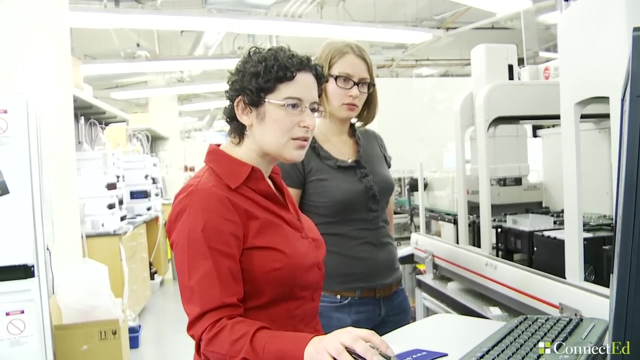 I looked at veterinary medicine for a while and eventually settled on wanting to study ecology. So I ended up doing laboratory research and focusing on fish physiology. I was interested in being a professor, but that didn't work out. so I started thinking about what I really liked about that job, About being a 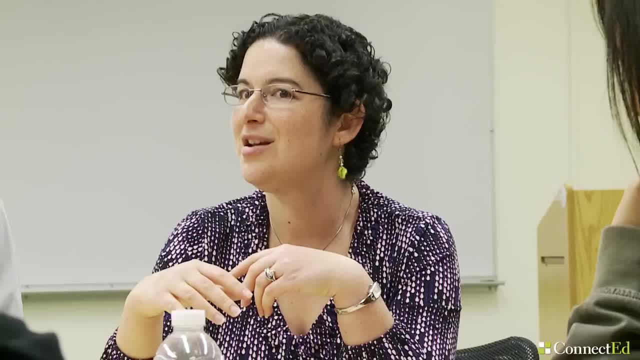 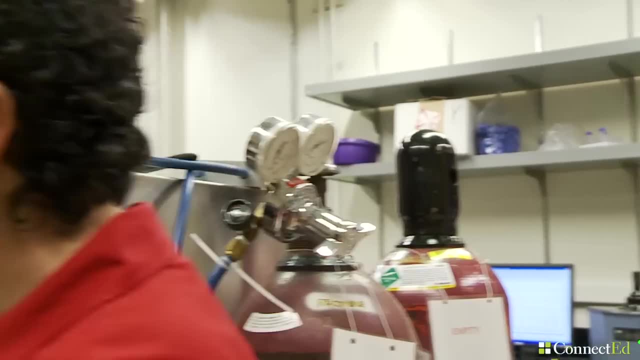 professor and it was working with students, It was working in a lab, It was doing a lot of mentoring and this job gives me a lot of what I was really excited about, So it's a very rewarding job As a female scientist. there are still definitely challenges Female scientists. 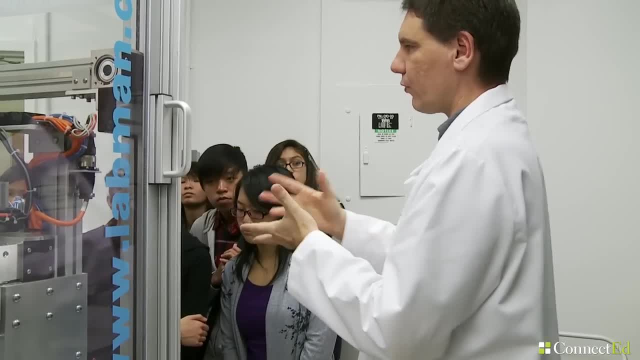 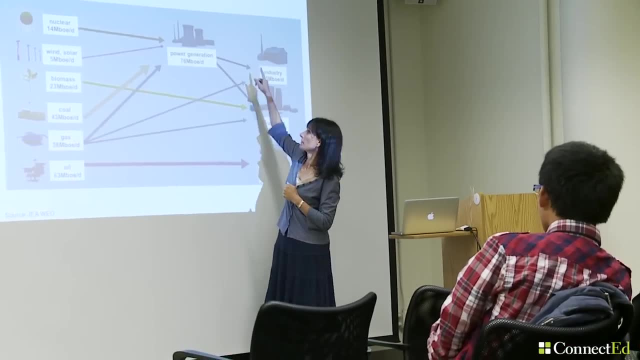 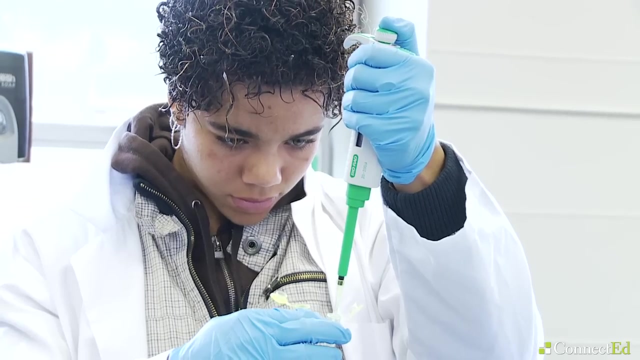 very often question themselves a bit more. because a lot of the models in science are built on male models, It's sometimes difficult to come in with the confidence that's expected, but at the same time things are definitely changing. So there's a lot more women in the labs now. For students that want to work in a 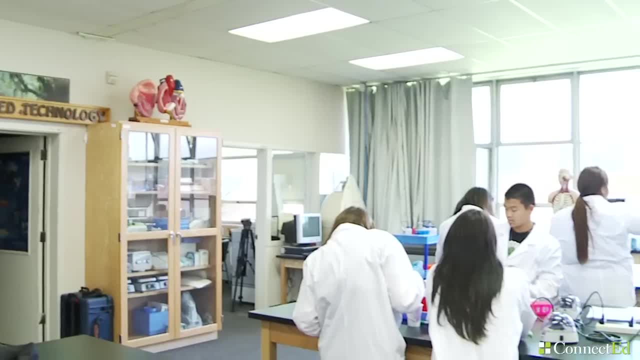 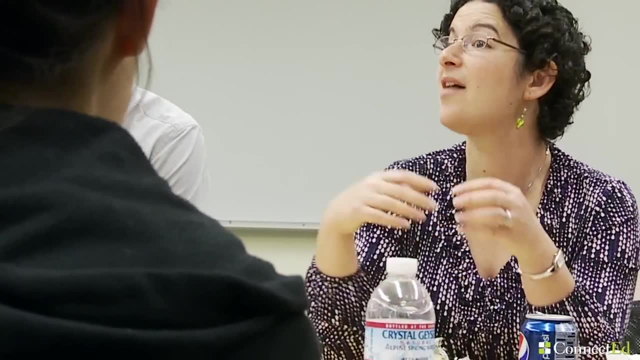 lab. my biggest suggestion is: it's never too early to prepare for a career in science, because you do need to take the science classes. You need to know what options are available to you, because I think high school and younger people are always asked: what do you want to do when you? 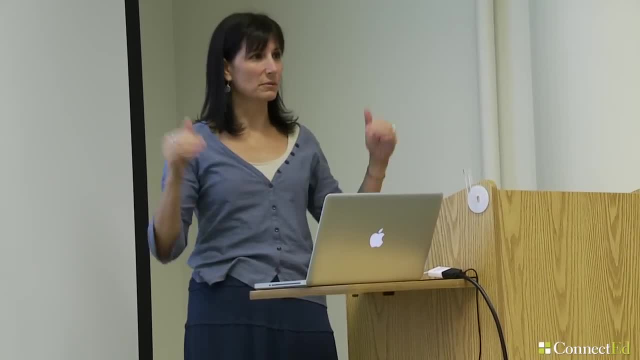 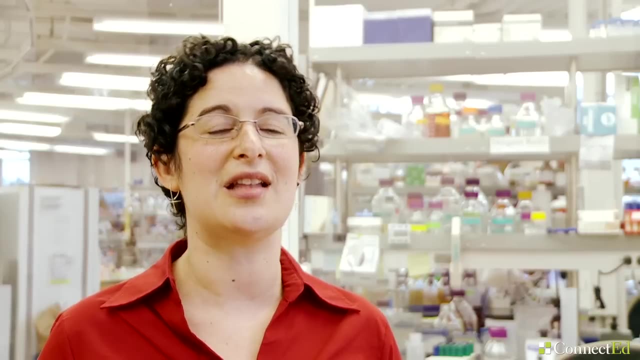 grow up. For high school girls who are looking into science as a career, make sure you find female scientists that can mentor you and to give you that support that you need. I think that's really important for for women who are interested in the sciences to find somebody that they can talk to you and